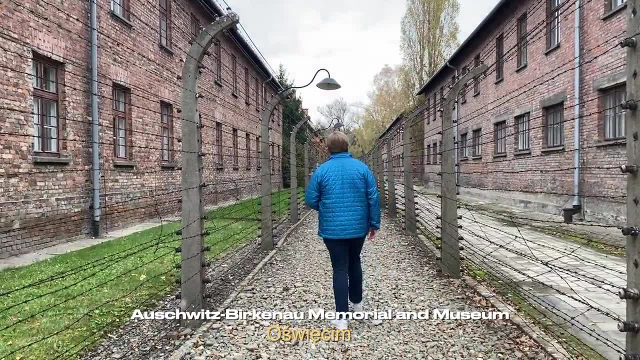 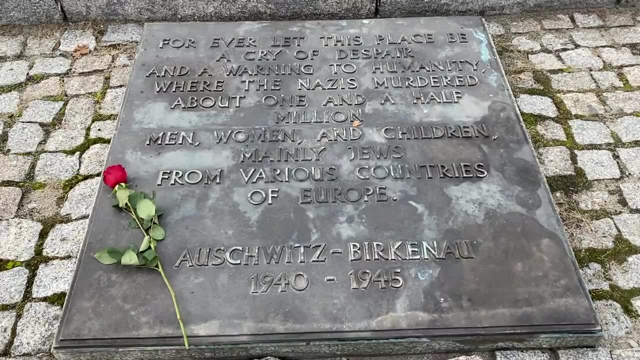 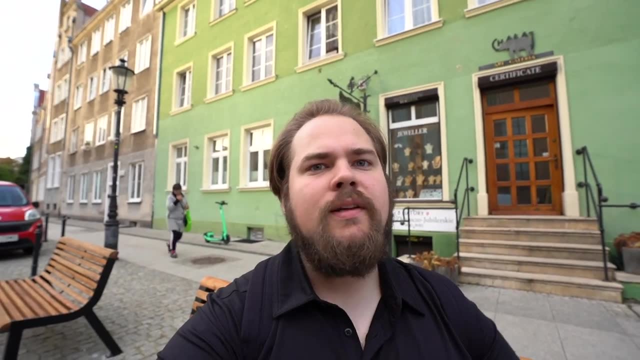 it's always the idea that we have to know what happened, We have to know how these events transpired, We have to know how it got to that point in order to make sure that that never happens again. This is one of those experiences where it's not gonna be enjoyable. It's not going to be entertaining at all, but it is something. 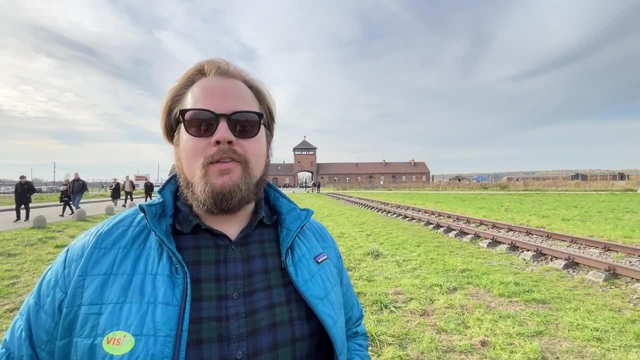 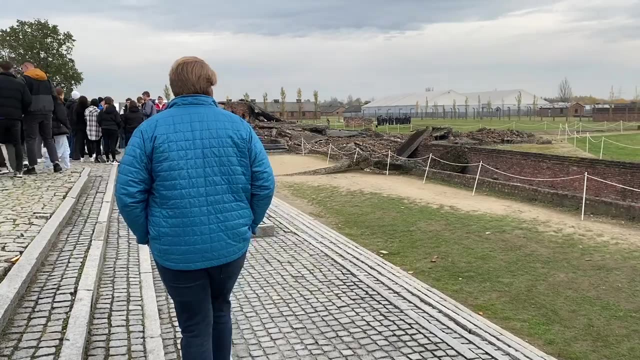 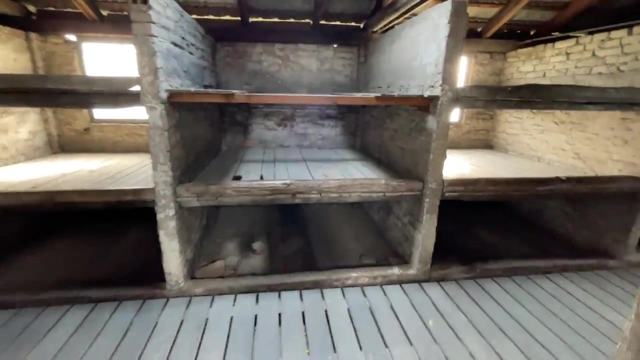 that's very important to do and it is a deep, powerful experience. We've just wrapped up our tour of Birkenau, which was the extermination camp. This is literally the train track that would bring people in to this horrific place. It certainly wasn't enjoyable, but I think it's really important for people, when they visit just this region of the world, to know that. 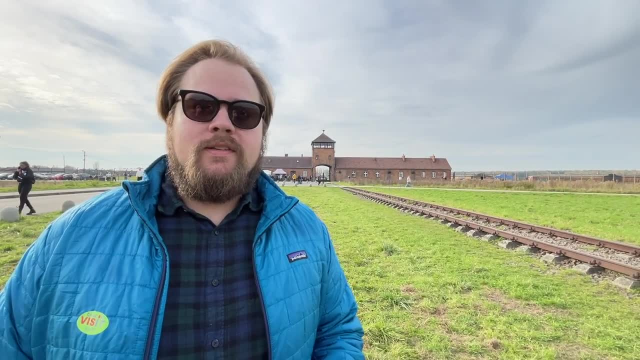 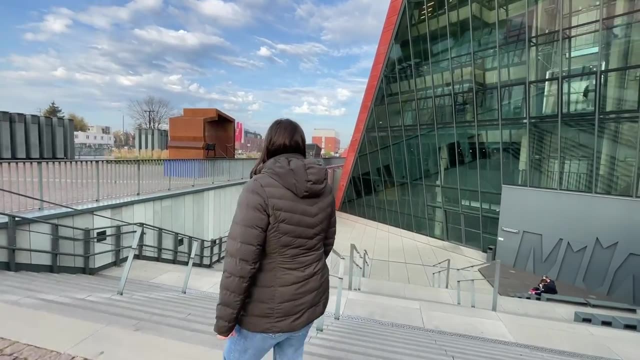 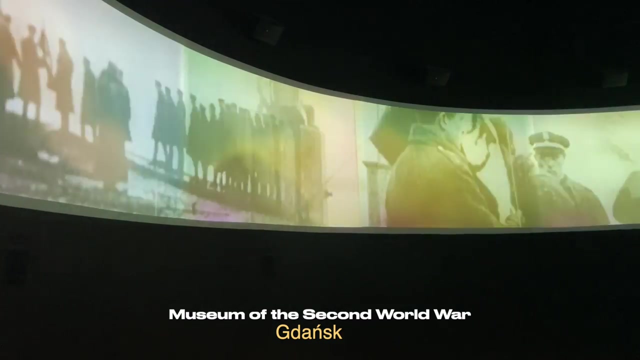 when this was occupied, everything kind of changed by the Nazis. This was literally death at an industrial level. It was a death factory. The World War II Museum right here in Gdansk is absolutely fantastic, Actually one of the best museums I think I've ever been to. when it comes to that kind of history, There's a 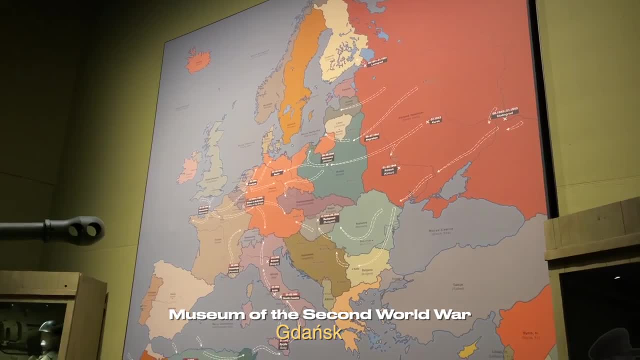 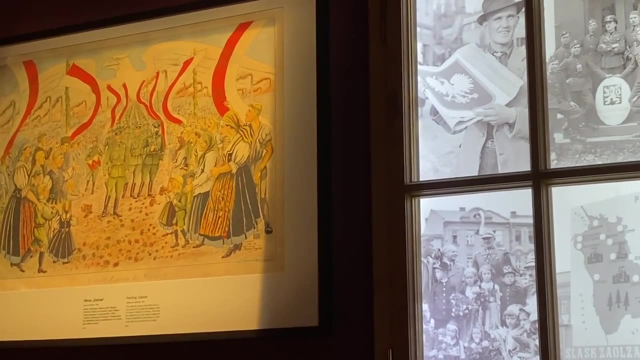 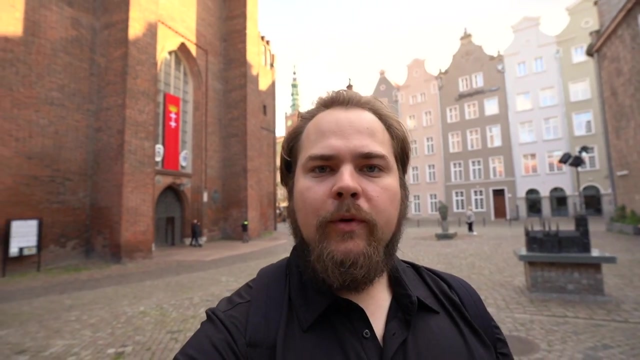 lot of information down there. This is going to take you a good two hours. We were down there for two and a half hours without even realizing it. There's so much to take in. Number three on the list is absolutely the prices. Poland is extremely affordable. 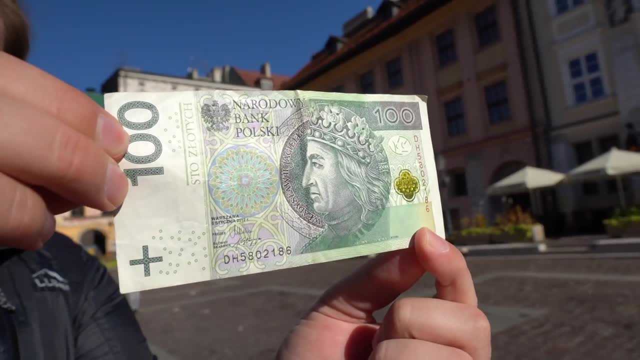 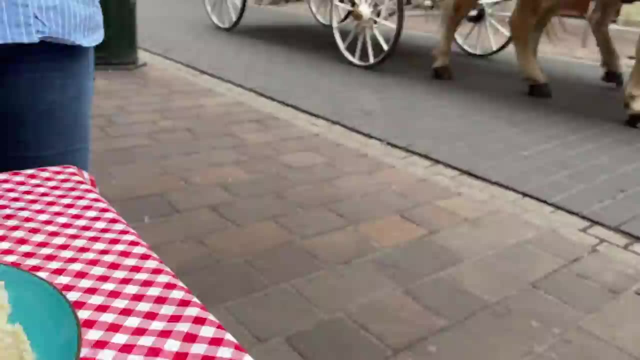 and I've talked about this on the channel before, but I think it bears repeating- It's not so much that it's a budget or a bargain experience, because when you have a budget experience, you're kind of expecting that the experience itself is going to suffer in order. 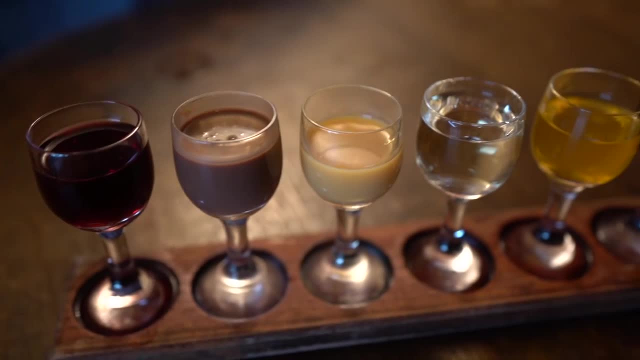 for the price to be lower. The thing with Poland is that, even though the prices are lower, you're going to get a very similar experience as you would in Austria, Germany, Switzerland, a lot of other countries in the world. You're going to get a very similar experience as you would in. 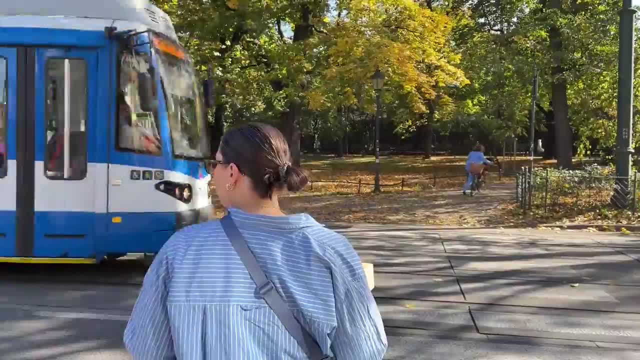 Austria, Germany, Switzerland, a lot of other countries in the world. You're going to get a lot of these places where you think of just the beautiful buildings. As far as the cities themselves, I think it's absolutely the best value in Europe. We've been to almost every European. 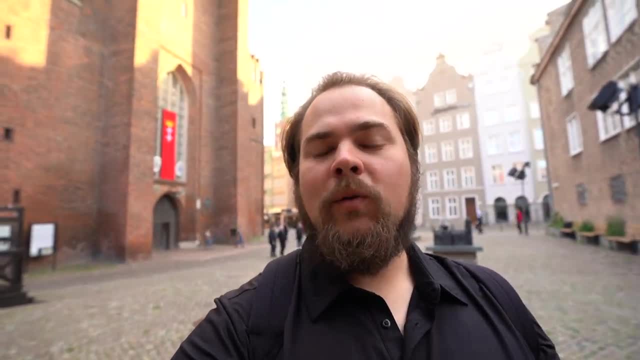 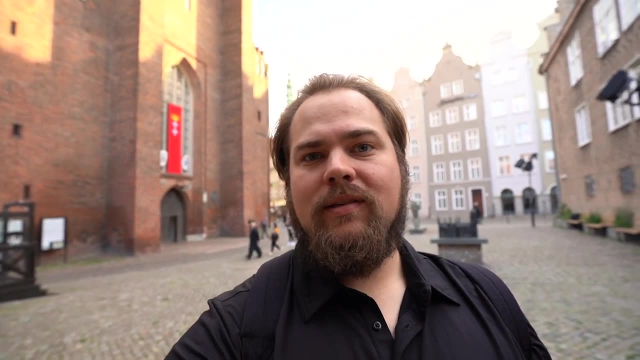 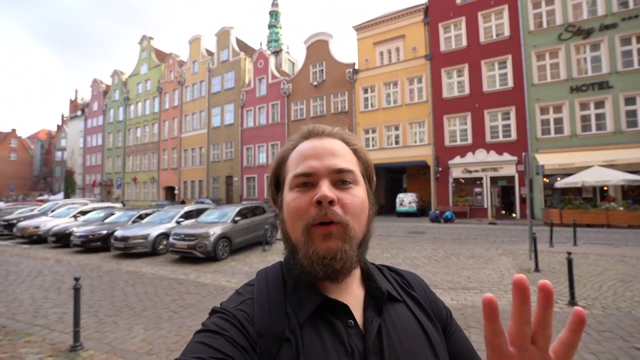 country, certainly on the mainland. I can say with absolute certainty: Poland is the best value you're going to find: Incredible experience, incredible cities for very affordable prices. The number four reason we love Poland- and this is a big one- is the food. The food here is absolutely. 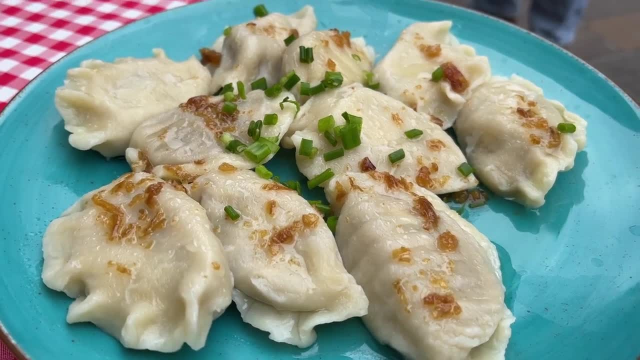 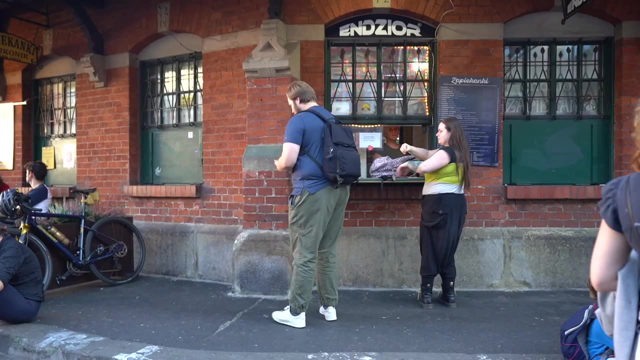 delicious Polish kielbasa, pierogies, potato pancakes, very rich food that's made with love and care, And this kind of goes hand in hand with the prices as well, because the fact that the prices are so affordable, that increases how much you enjoy the food. experience A lot of these restaurants. 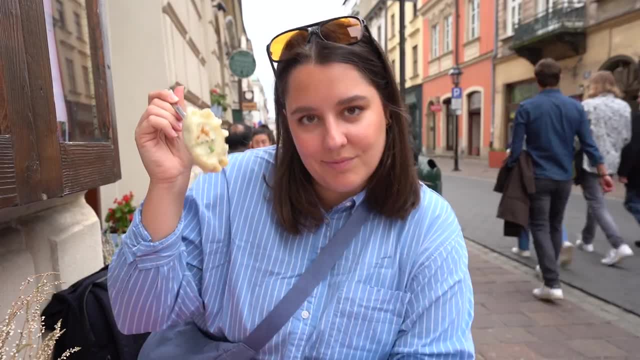 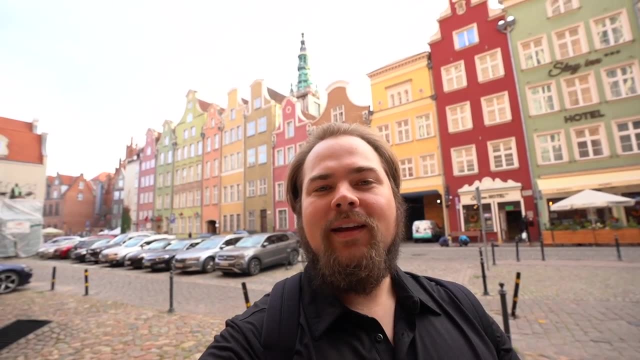 we've been to, we just have an incredibly delicious meal and then the bill comes at the end and we're like what really? It's hard to believe sometimes, But Polish food, Polish cuisine, is absolutely a reason just right there to visit this place. It's a great place to visit. It's a great place to. 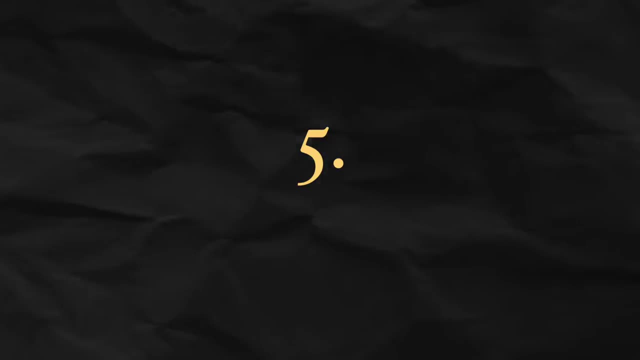 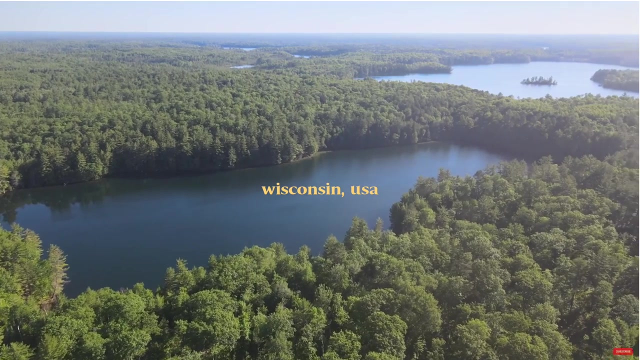 visit. It's an amazing country. The number five reason we absolutely love Poland- and this one might be the most controversial- it's just the seasons, And I think, for me personally, it's just because it reminds me of home. I come from Wisconsin, I come from the Midwest, and we just 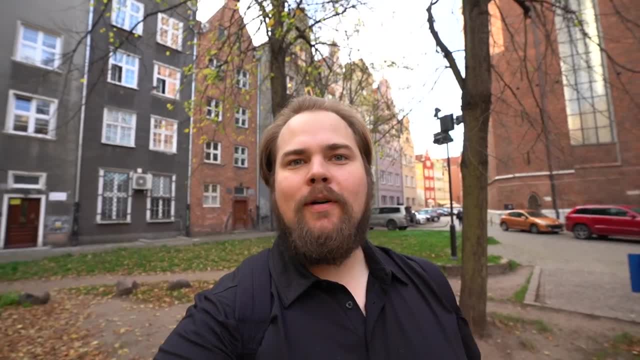 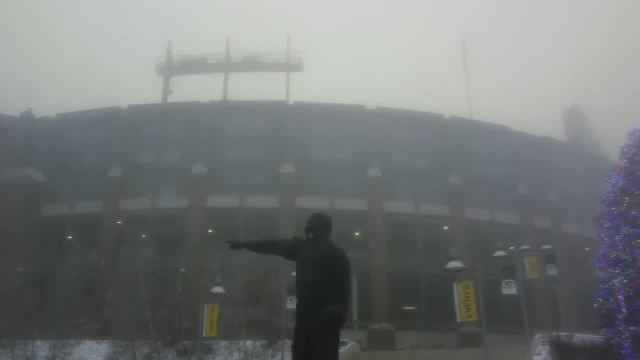 love the fact that we get four seasons. Yes, I know all you California people love to just have perfect weather every day, but personally I love the changing of the seasons. I love fall, I love winter, I love snow on the ground during Christmas And we're here during fall, as you can hear, the 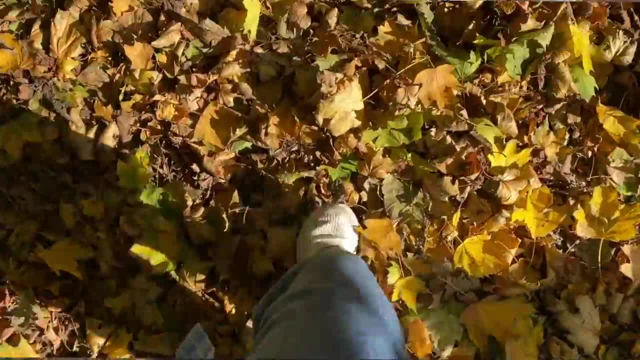 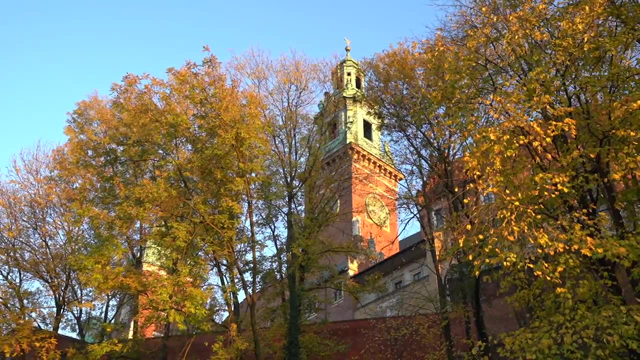 leaves crunching beneath my feet, and it has been just an incredible experience. I love the experience. In Krakow there's this amazing park that goes all the way around the old town, and seeing all the leaves change as we walk through that park, it was truly breathtaking- And I'm a 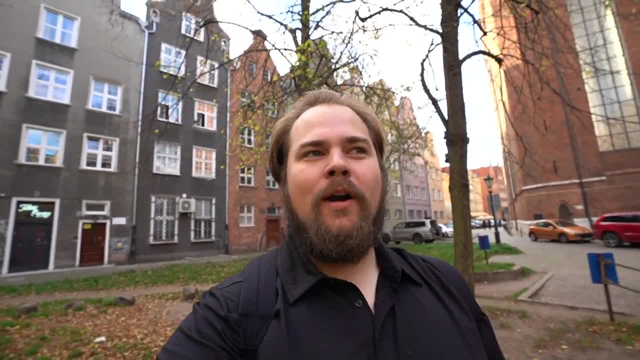 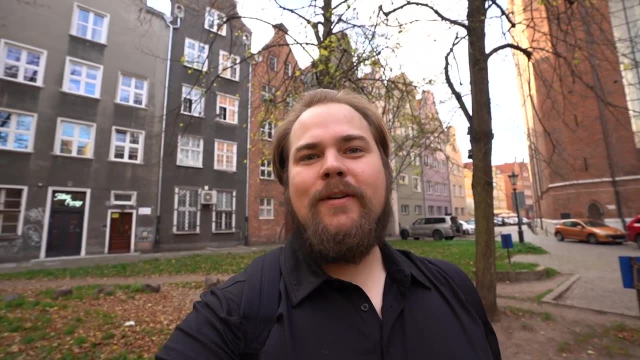 big fan of fall, So coming here during the fall has made me love Poland even more. Now, of course, the one negative there is that the winter is pretty unpleasant, But again, I'm a Midwesterner, I'm used to that. If you come during the fall, if you come during the summer, it's a beautiful place. 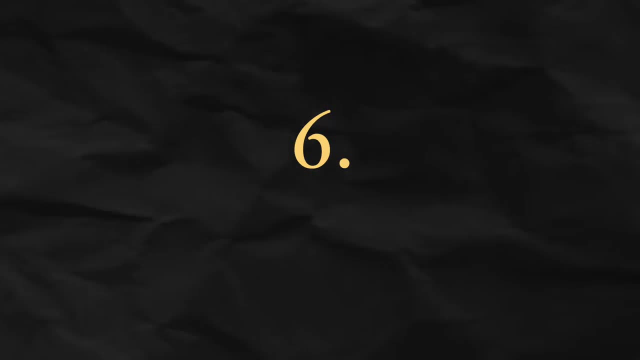 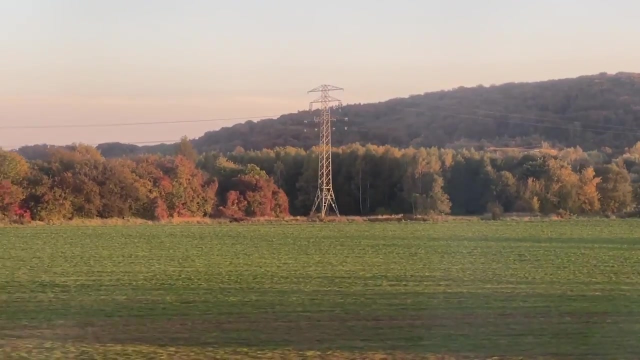 to be Number six on the list of the reasons we love Poland is the convenience. It's a very convenient country When you go to the airports. when you go to the airport, you can go to the train stations. There's ways to get around. In Krakow they have a streetcar and in fact it's 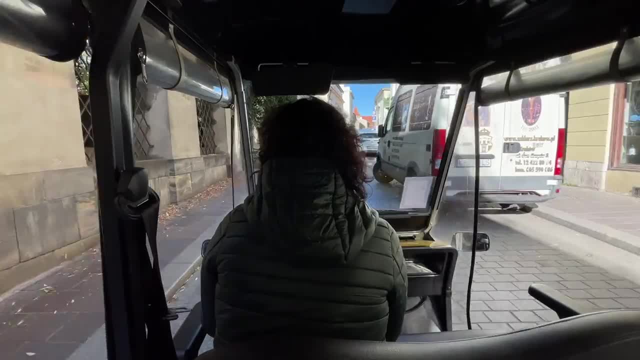 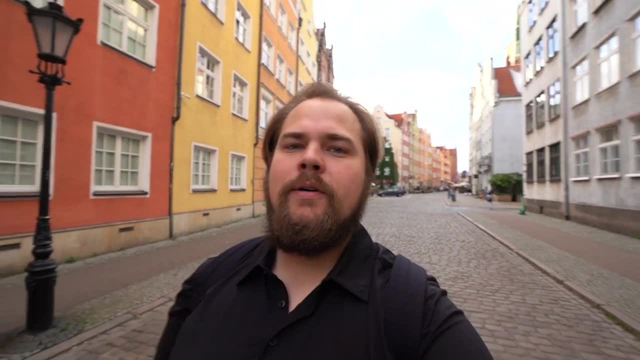 mostly walkable, The directions are not too hard to figure out and people are always helpful if you're not really sure where you're going. We've been to a few countries where you know you can easily get turned around, and I think Poland is definitely not one of those countries, because 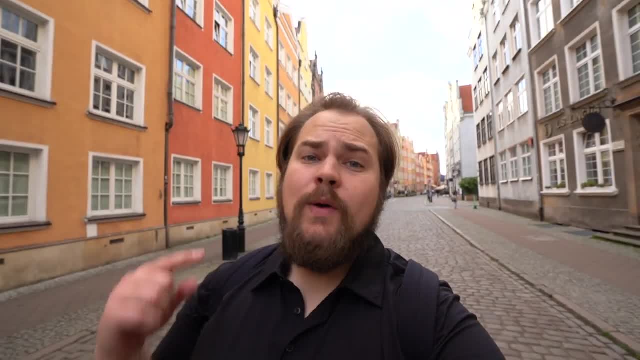 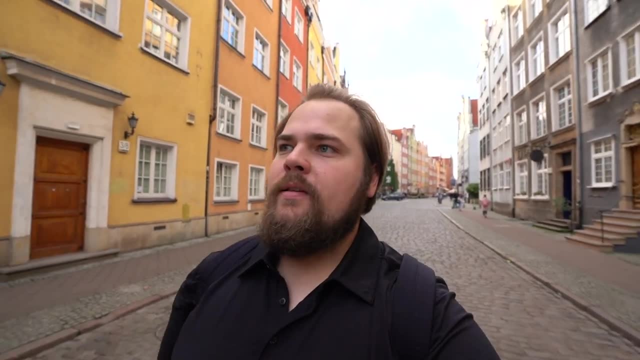 there's just easy, convenient ways to get around. They also have Uber, which is a big thing. Uber is not guaranteed in every European country, so the fact that they have that here is a big plus And I think just in general, it's very easy to get around. All the cities are well-connected. The 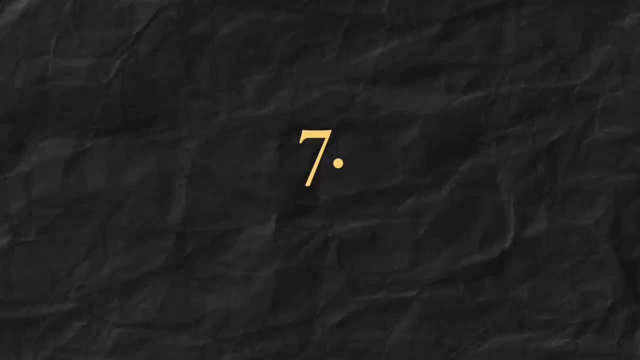 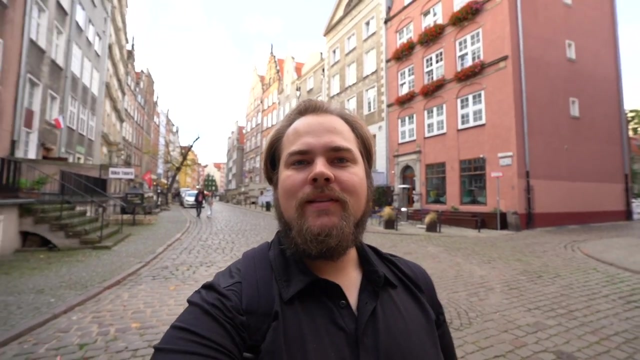 trains are nice. The trains are very modern and clean. And finally, the last reason, the number seven reason we love Poland is the people. People are so friendly. here in this country We've had a few instances where people just help us out without even us asking. Everyone here speaks. 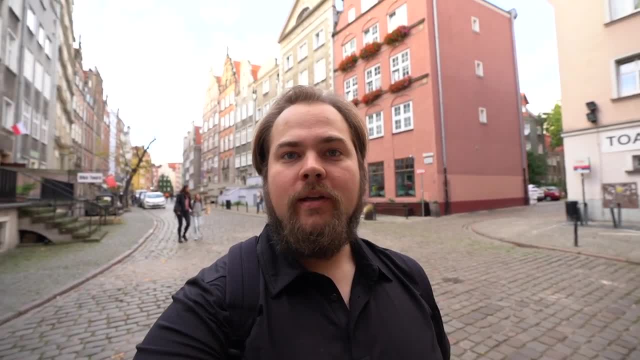 English. That's becoming more common in Europe, basically everywhere, but here especially, the English is superb, literally fluent. everyone you talk to And just overall it feels very welcoming. It feels like people want you to know that you're here, that you're here, that you're. 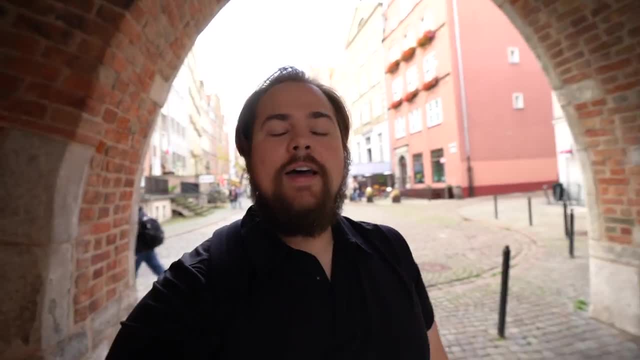 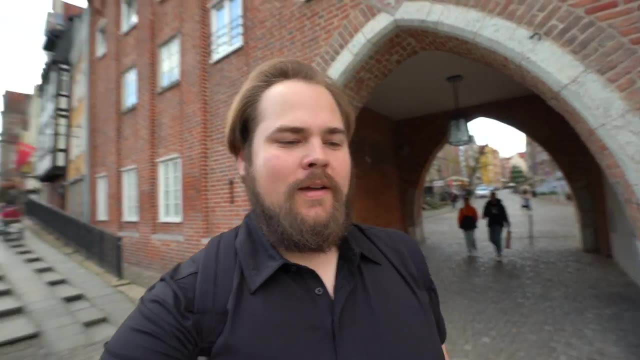 here. They're excited that you're visiting their country and that I absolutely love, because that's how I feel when people visit my part of the States. So I really love the fact that you can go pretty much anywhere here in Poland and people are going to be very friendly to you If you say. 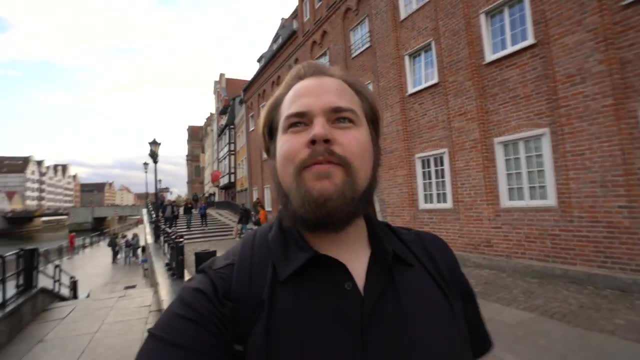 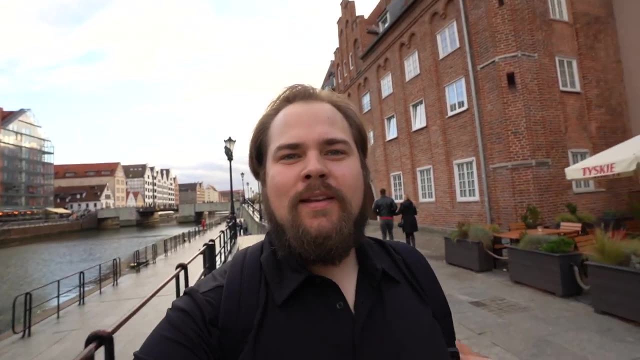 do you speak English? they will. You don't have to worry about it, but it's polite to just ask first. And even a few words in Polish, if you do get them down, makes it a little bit easier. This is a place we knew we had to add to the list and we're so glad we got here. 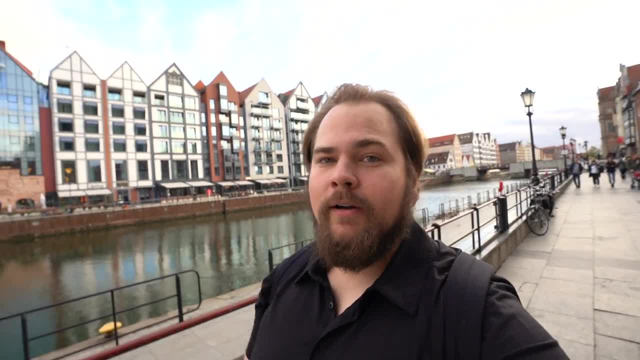 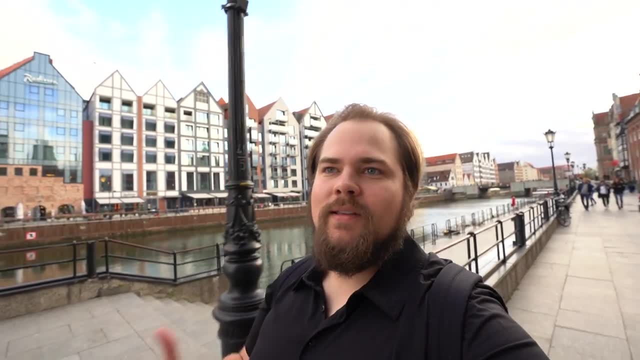 Even though it ended up being towards the end of the year, it might be our favorite country, If you just take in all of the factors. Now, of course, if you go to Switzerland, if you go to Italy, if you go to France, if you go to the south of France, if you go to Greece, a lot of these places- 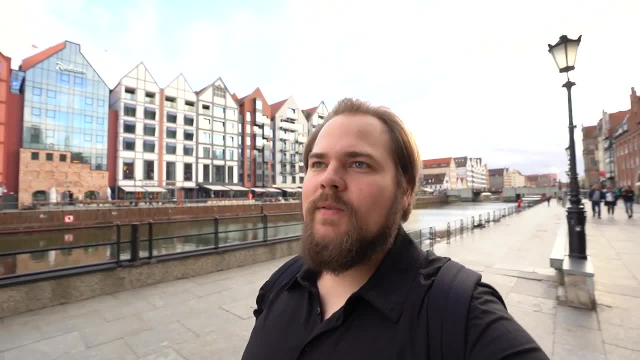 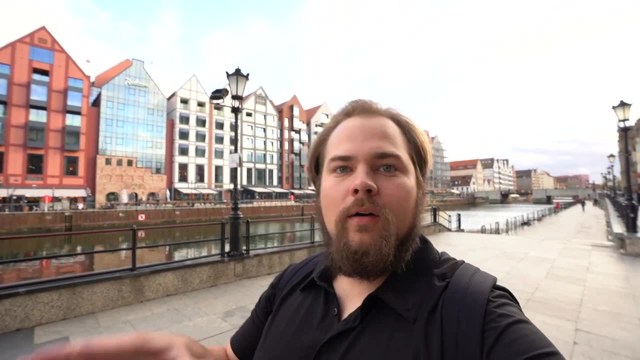 are luxurious and beautiful, but the thing is you have to factor in the prices how affordable it actually is to go there, and you have to factor, like, how people treat you when you're there. And I think when you factor all of those things, Poland is definitely near the top. It's the best. 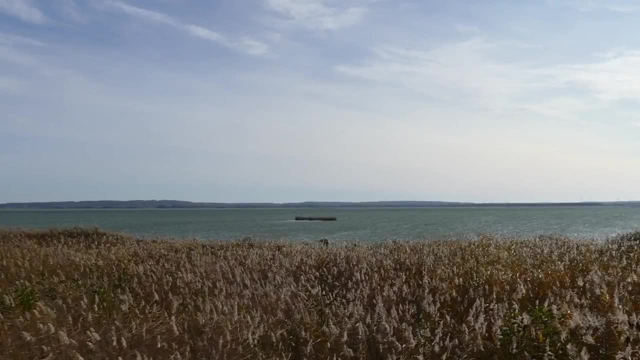 value in Europe. There's no doubt about that In my mind, And we're going to have to come back here because, again, we still haven't even seen the capital, We still haven't even seen Warsaw. So this definitely won't be our last time in Poland. 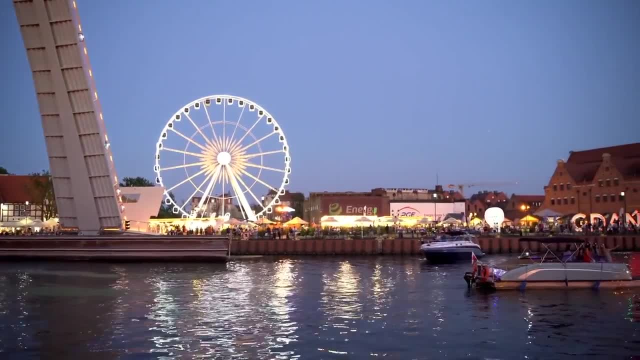 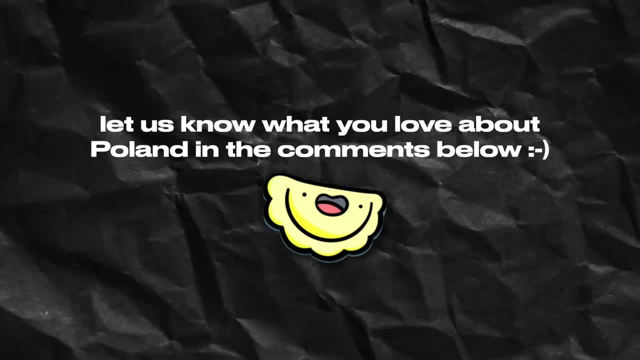 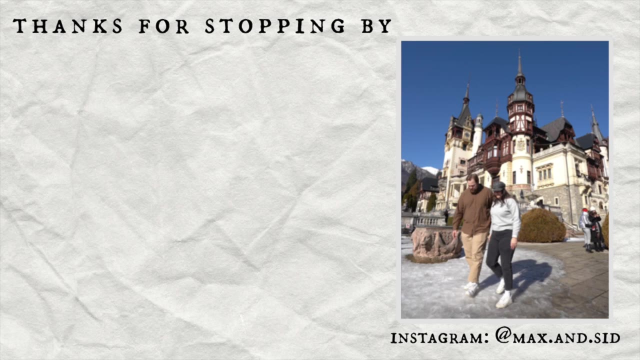 I hope this inspires you to visit Poland as well. Thank you so much for watching. I'll see you in the next video. Bye-bye.